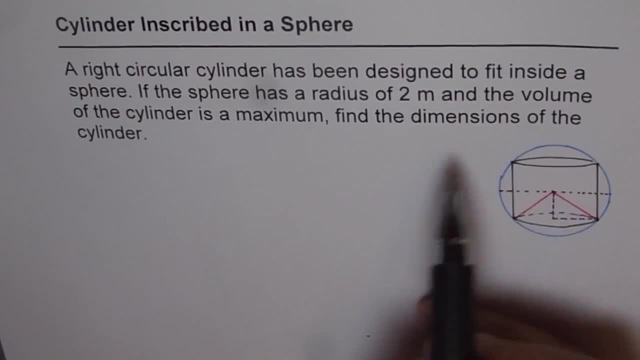 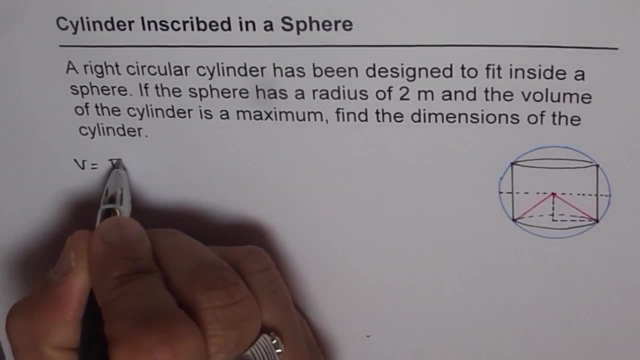 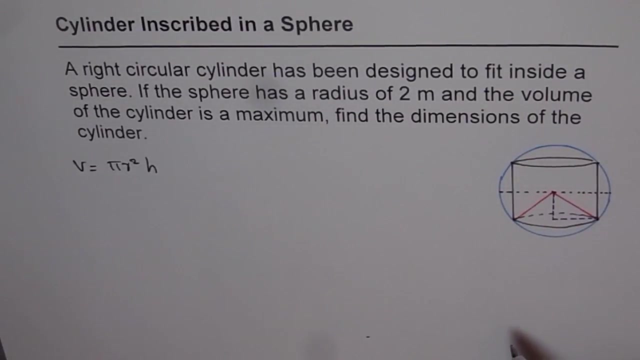 to be found. Now here we want to find maximum volume of a cylinder. Now, volume of a cylinder is given by pi r square, h right, Where pi r square is the area of the base and h is the height of the cylinder. Now we are also given here that it is inscribed within a sphere whose radius is 2 meters. That means from center to the edge this line will be 2 meters. 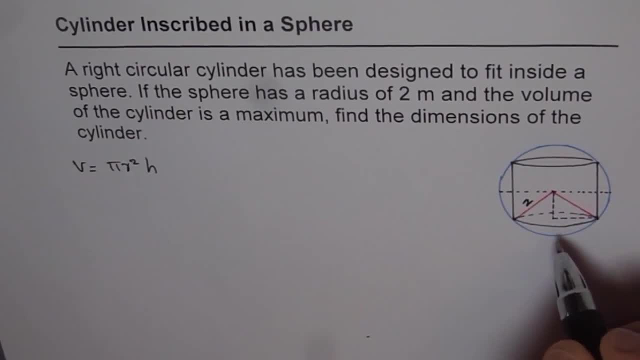 So, and that will help us to find a relation between radius and the height, correct. So what we will do here is we will try to find a relation between the height of the cylinder and the radius of the cylinder. In that case we will have our equation in one variable. At present we have it in two variables. So let this be the radius r and that is the height, I should say half. 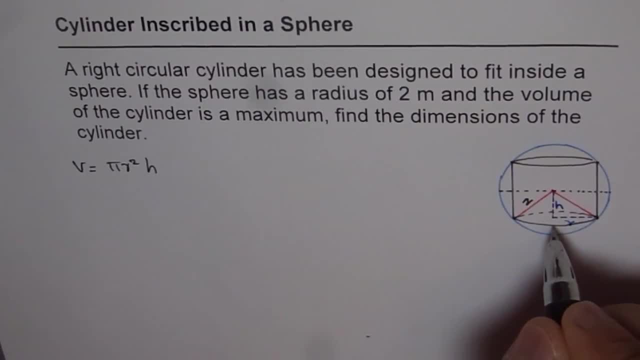 of the height right. So this is half of the height of the cylinder right. Let me write this as h over 2 and I am writing this as my height of the cylinder right. Okay, So now we have a right triangle here. So from this right triangle we can find a relation between height and radius, correct. So we get h over 2 whole square. 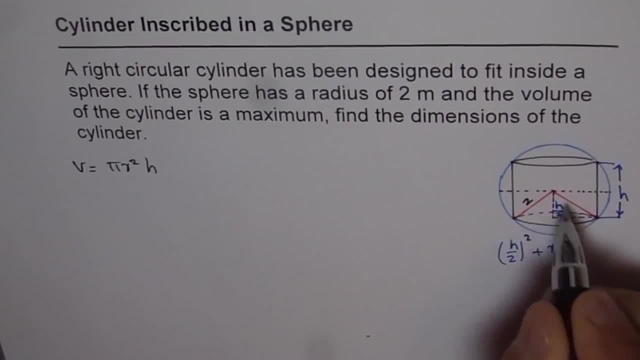 plus r square equals to the hypotenuse square, which is 2 square, right? So now we have a relation and from here we can find what r square is in terms of height. So we need r square. It is better to find r square from here. So we get: r square equals to 2 square is 4 minus h square by 4, correct? So that is the value of r square. So we will substitute this value in our equation. 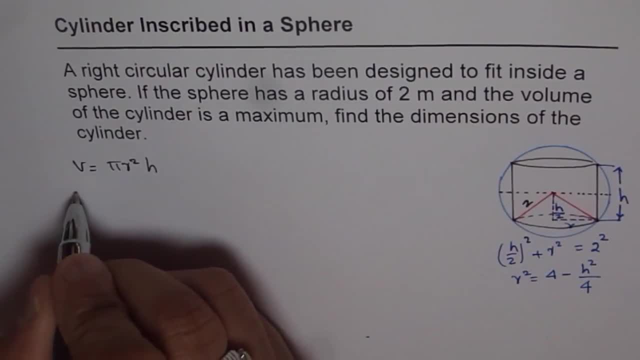 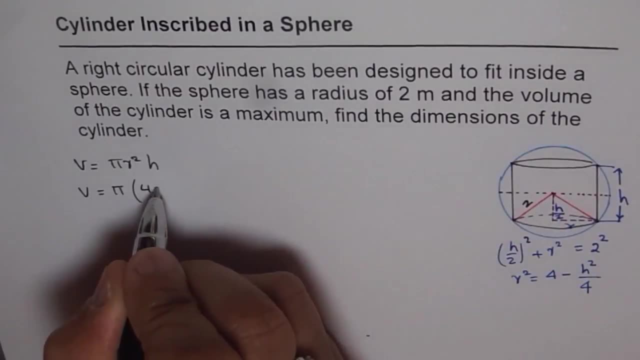 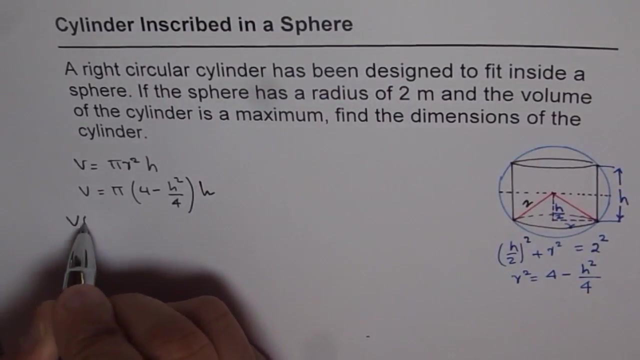 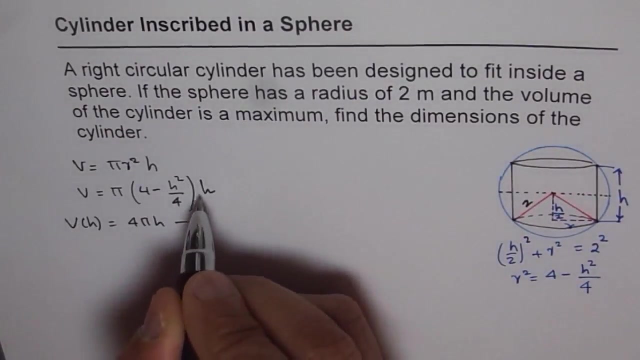 We will substitute this value in our equation for volume and then find the rate of change of volume. So we have now pi and r square. we found as 4 minus h square by 4, and that is times height. So now we have volume in terms of height, correct? So we can now open the bracket and we get 4 pi h minus. so it is pi h cube over 4, correct. We will multiply with this. 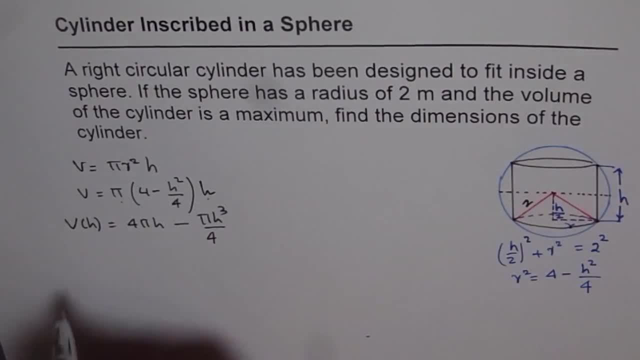 and this both the terms inside. Now the derivative of volume with respect to height is 4 pi, and this will give us minus 3 pi over 4 h square. Now to get the maximum volume we need to find the critical number right. So always critical number is when this derivative 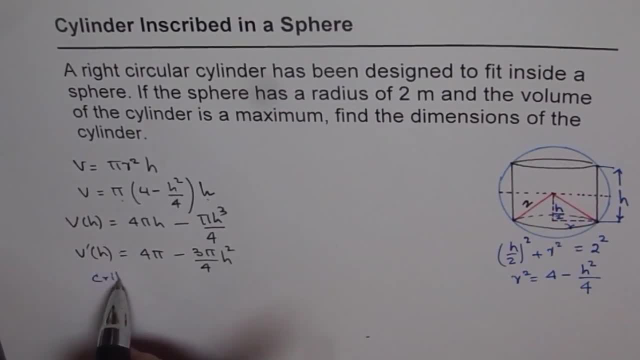 is 0, right. So let's find the critical number. that is, we'll equate v dash h to 0.. So we get 0 equals to 4 pi minus 3 pi over 4 h, square right. So that is how we can find the critical. 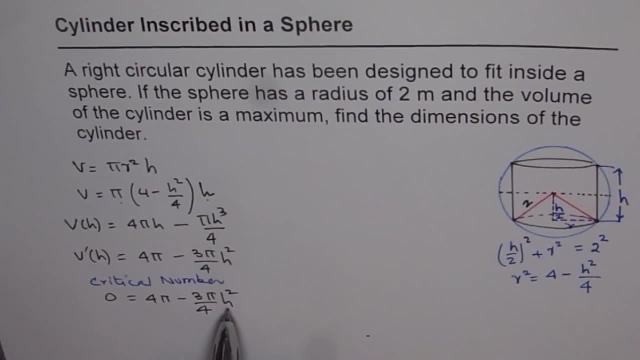 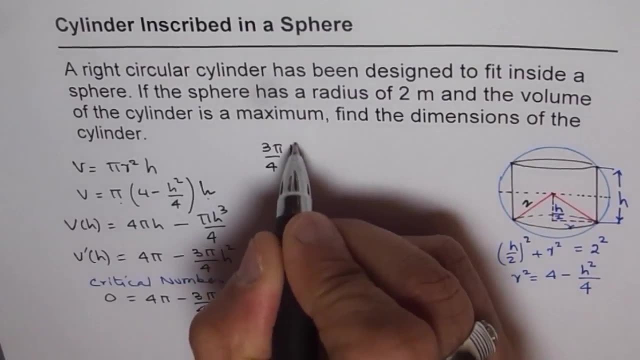 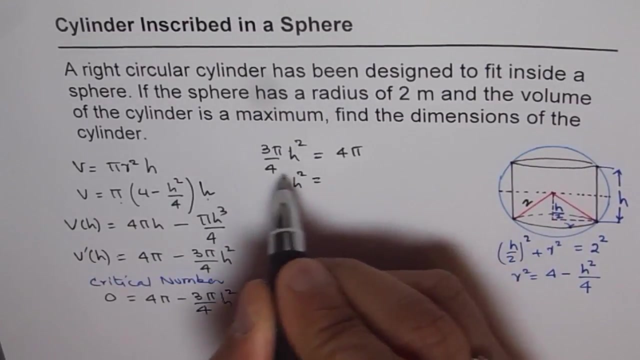 number. Now here let's try to find what is the value of h. So we have 3 pi over 4 h square. h square equals to 4 pi. Let's isolate h from here, So h square equals to 4 times. 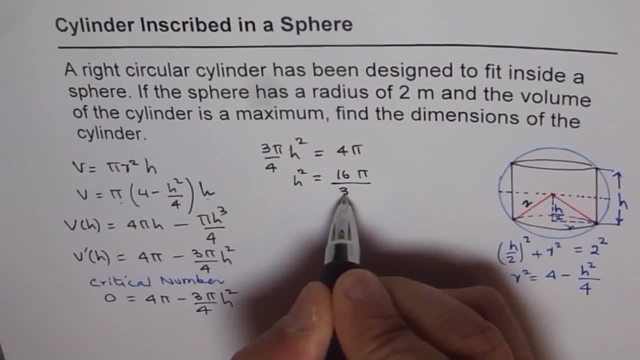 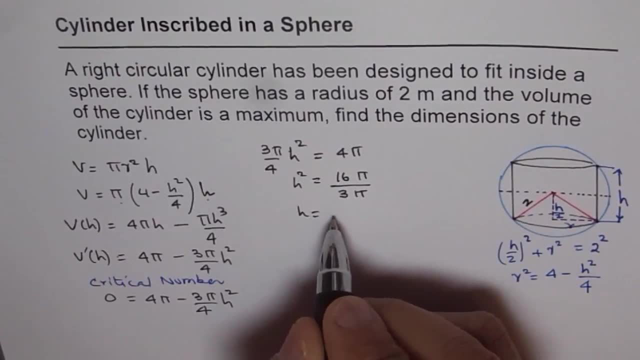 4 is 16, pi divided by 3, pi, right And h will be equals to square root of this. Square root of 16 is 4.. So we get 4 over square root of 3, right Pi and pi will cancel out correct. 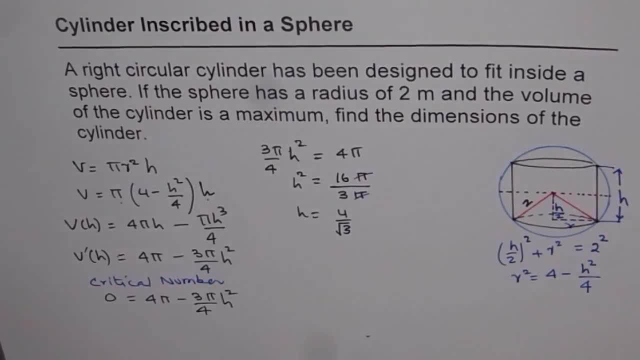 So once we do square root, pi and pi will cancel out and we get height as 4 pi over 6 pi over square root of 3. And for this particular height radius will be. so we can substitute this height here and find radius. So we have h square. we can substitute 16. 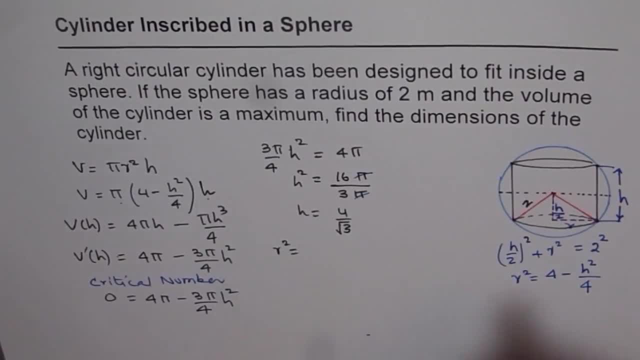 over 3 there right. So we have: r square equals to 4, minus h square is 16 over 3.. So write 16 over 3.. That is h square divided by 4.. That is this correct. So this can. 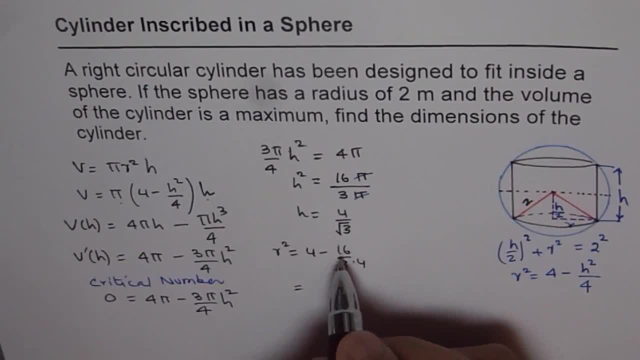 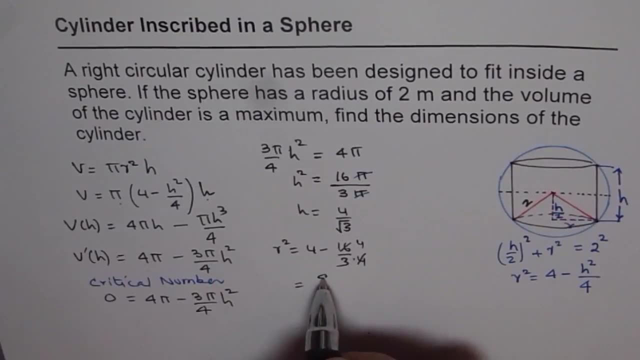 be simplified and we can now write this as this is. this goes: 4 times 4, pi over 16 over 4 over 3 here. so 4 times 3 is 12 and 12 minus 4 is 8, so we get 8 over 3 and r will be square root. 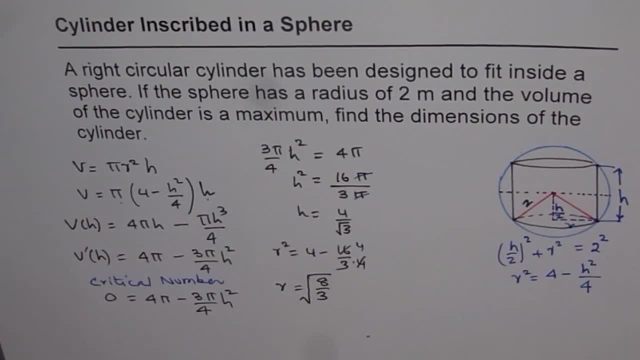 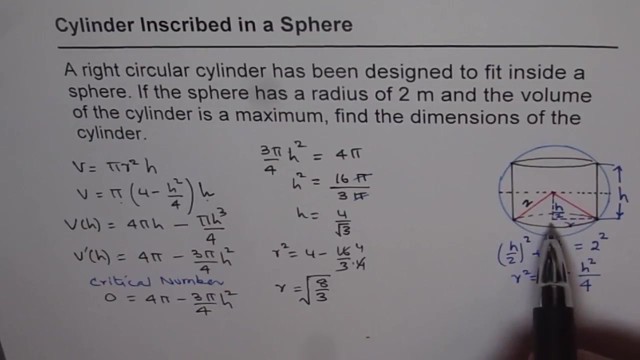 of 8 over 3.. So that is how we can get height and radius for this critical number. Now we have to prove that this critical number indeed is a maximum. Now, to do that, what we should do is we should find what are the restrictions on this height right? What can it be? Since we are in a 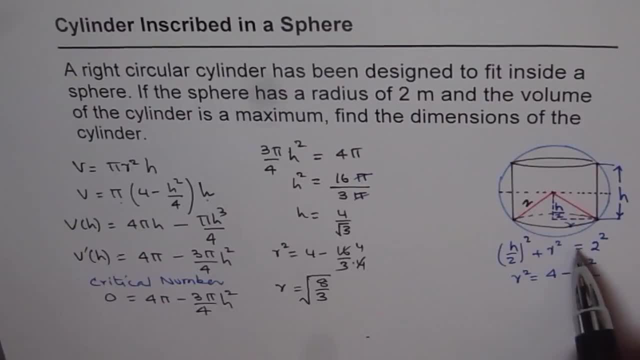 sphere of two radius of two meters, so the height could be maximum four meters, correct? So we have here that h actually could be greater than equals to zero, but less than equals to four. That is the limit, right. So let's find the value of volume for these critical numbers. 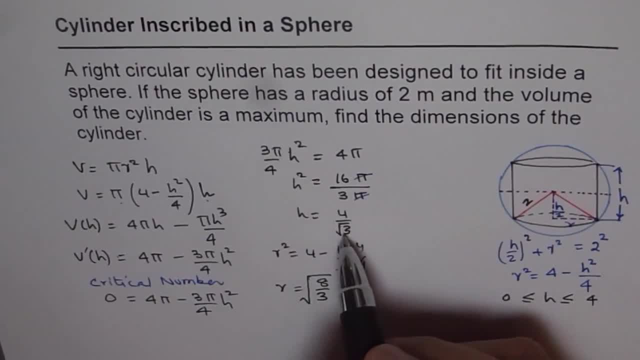 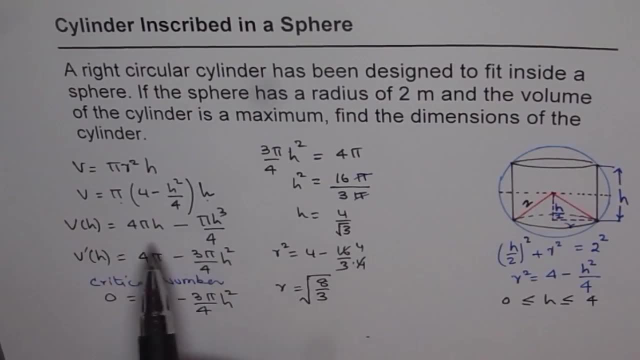 Right. so we have critical numbers 4 over square root, 3 and 0 and 4.. So we'll plug in these values in our expression: vh equals to 4, pi h minus this right, So we can use this one of these equation to find the best possible answer. Now, let's say so. let me just demarcate these so that you know. 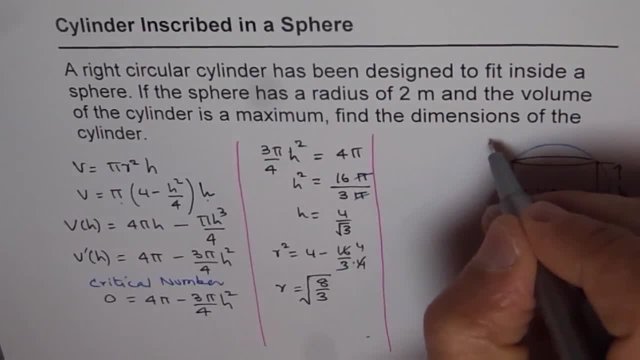 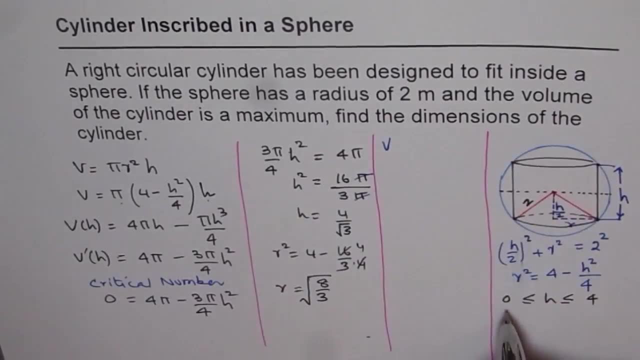 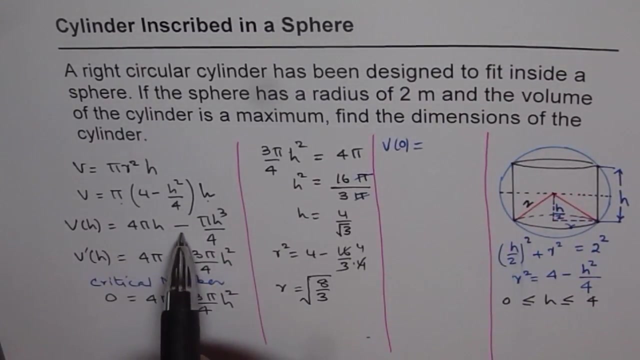 clear about what has been done and where We have some space to work right. So now what we will do is we'll find volume for critical number zero. So volume for zero is equals to. So we can use one of these equations: So it is 4 pi h minus. 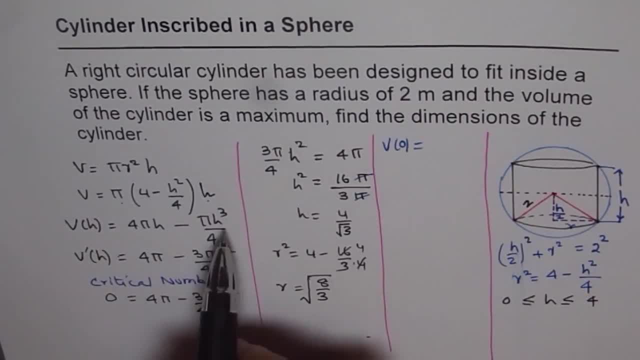 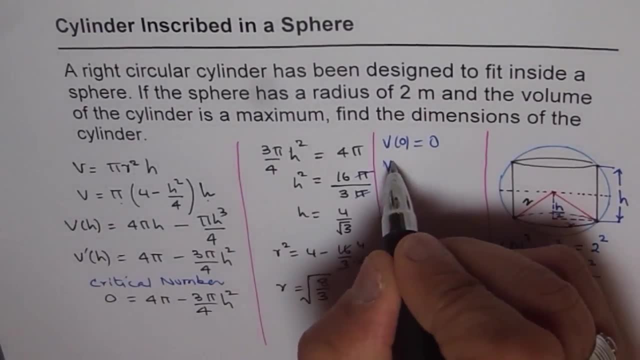 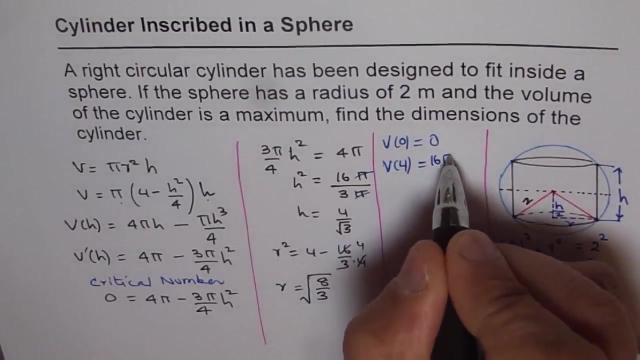 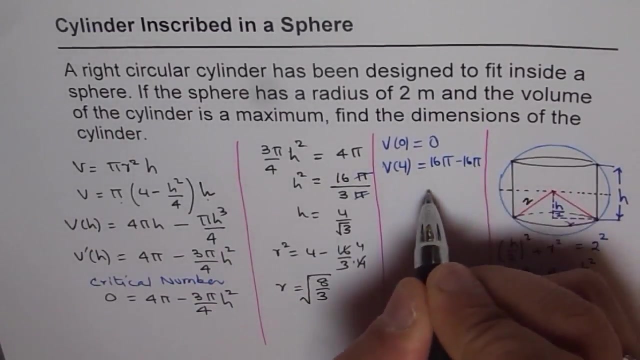 pi, h cube over 4.. So if I put h as zero, then of course this will be zero, right. Now for h as 4, so that means volume at 4.. We'll write 4 here, so we get 16 pi, and 4 here, So 1, 4 will cancel, So we'll get minus 16 pi, which is also zero, right. 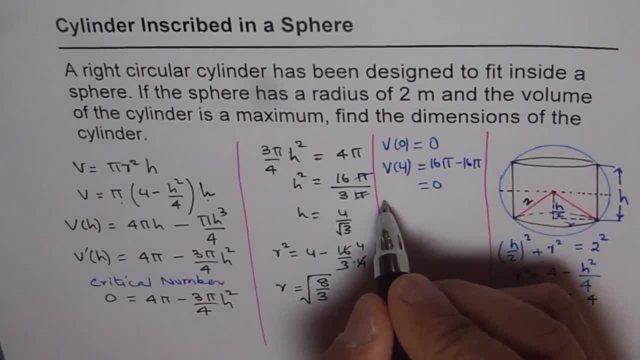 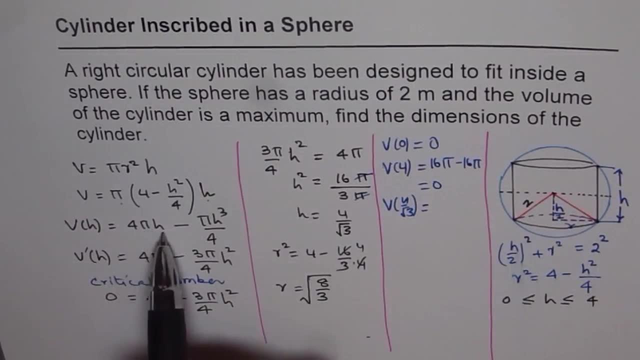 Now the third value is 4 over square root 3. So volume for 4 over square root 3 is equals 2. So when I write 4 over square root 3 here, I get 16 pi over square root 3.. 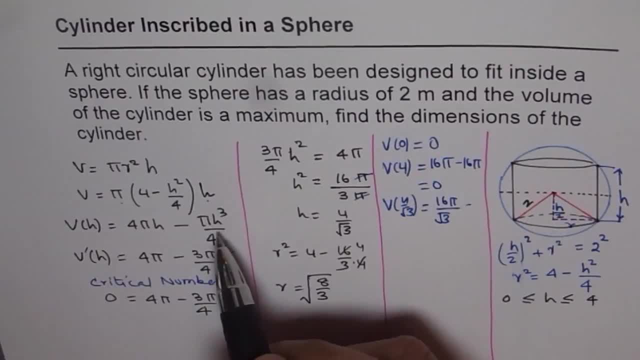 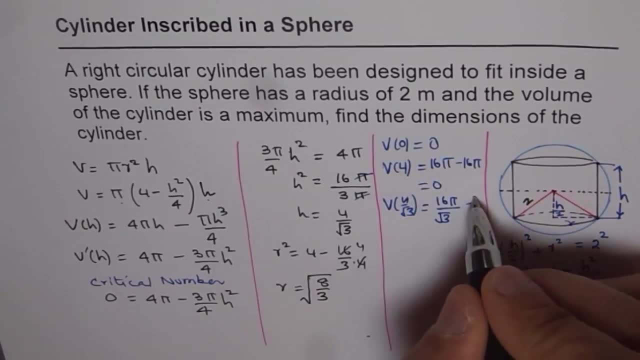 Minus now 4 over square root 3.. So 4 cube. one of the 4's get cancelled, So we get 16 pi 4 over square root 3.. So 4 over square root 3.. So square root, 3 cube. So that is what. 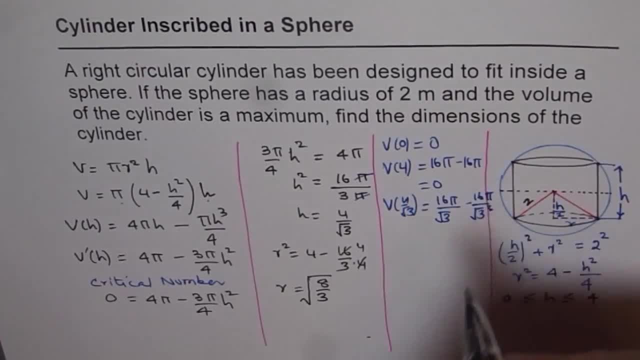 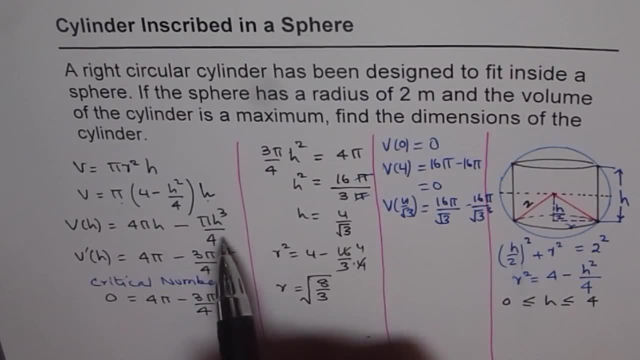 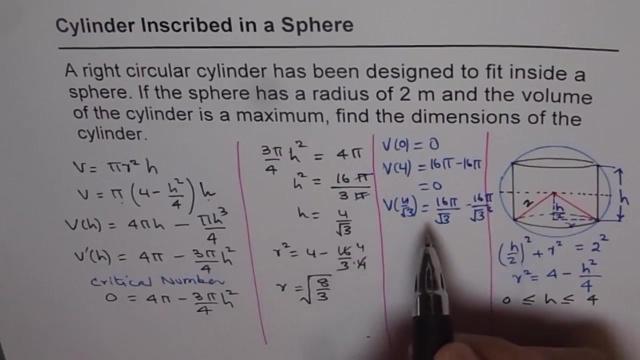 we get here Times pi, of course, right. So what I'm trying to do here is I'm trying to write the value 4 over square root 3 here, right? So 4 cube. Ok, let's do it again. So we have 4 pi. So first we put in this: we have 4 pi times h is 4 over square root 3. ok, Minus. 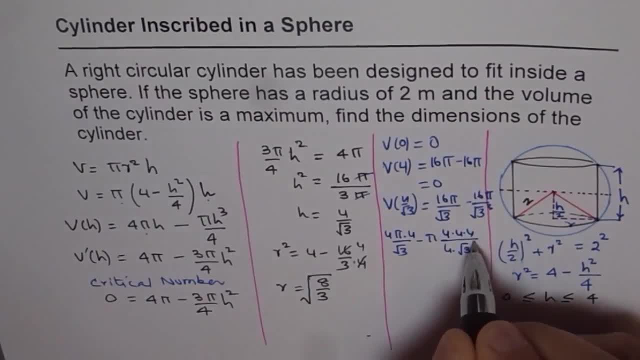 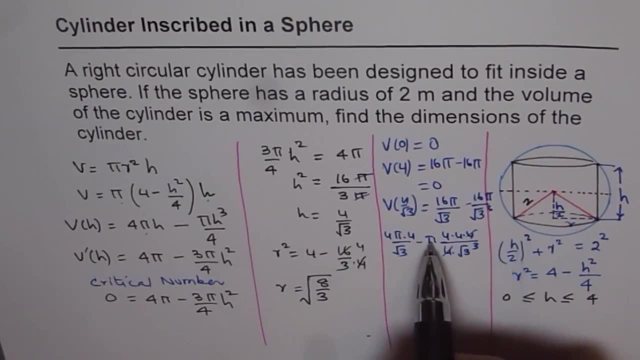 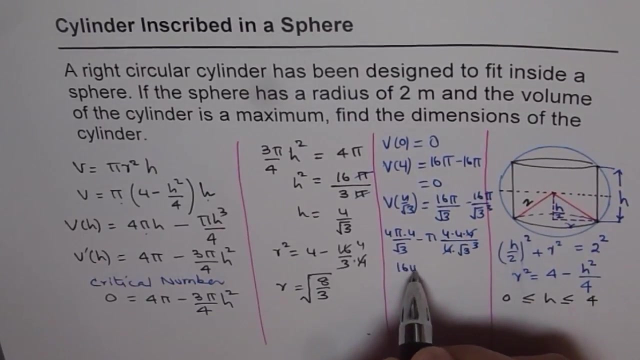 1, 4 times square root 3. cube Correct, That is what we have written here. So one of the 4's get cancelled. What I'm trying to say is this: So we get 16 pi common factor. So we get 16 pi over square root 3 as a common factor. So we get 16 pi over square root 3. 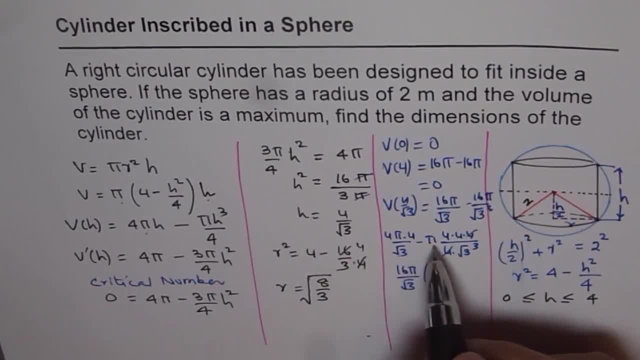 as a common factor. And then we get here our volume as 1 minus 1 over 3.. Minus 1 over 3. Right, 1 minus 1 over 3. Because 3 square is remaining Right, So we get 3 over 2.. So 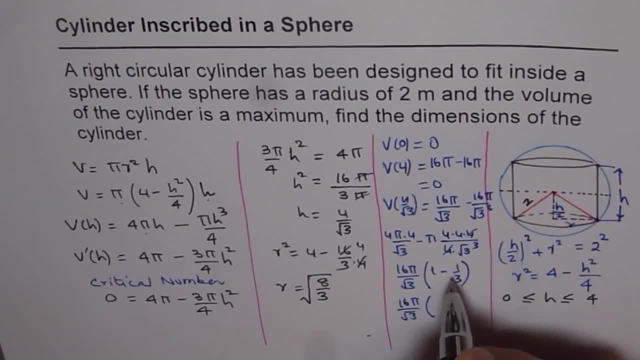 we get 16 pi over square root, 3 times 3 over 2.. 3 minus 1 over 3, which is 2 over 3.. So clearly this is a positive number. right? Since this is a positive number, here we have maximum. 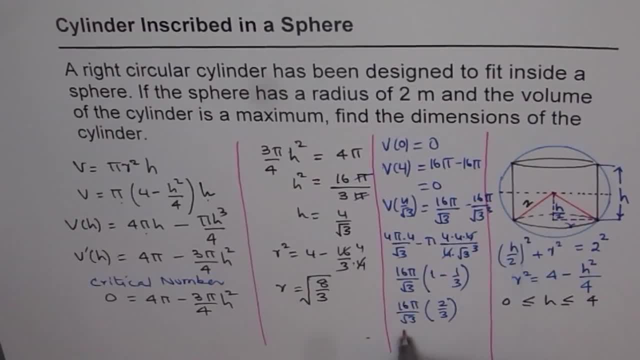 So the critical point which we found indeed gives us the maximum value Right. It is kind of very important to show that, show these calculations and say, well, we have a boundary condition and we have checked all the values, that is, at the boundaries and at the critical number and amongst all those values.